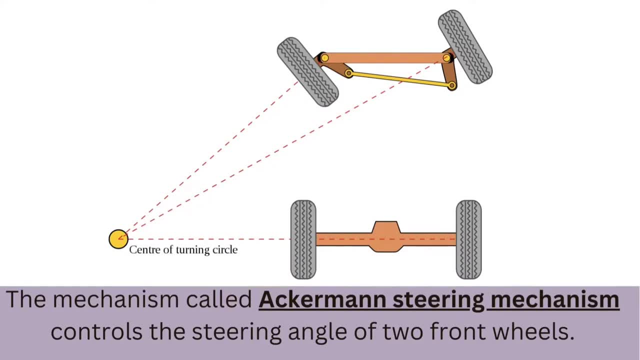 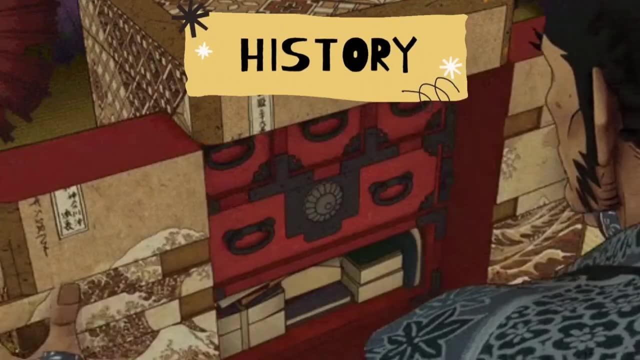 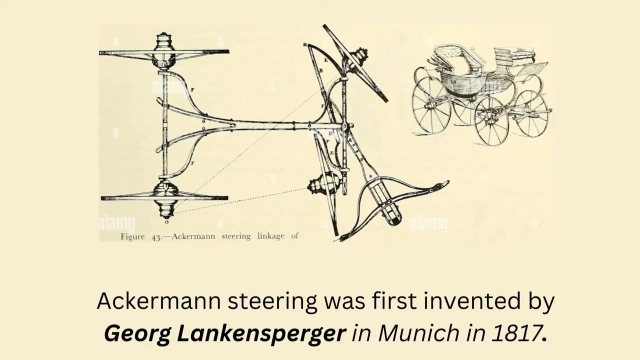 The mechanism called Ackermann steering mechanism controls the steering angle of two front wheels. Let's see the history behind the Ackermann steering mechanism. Ackermann steering was first invented by Georg Lankensperger in Munich in 1817.. 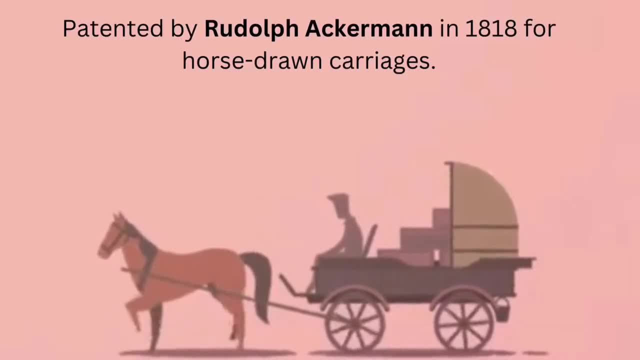 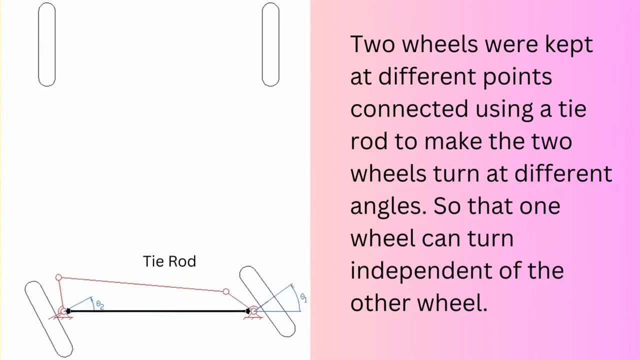 It was then patented by Rudolf Ackermann in 1818 for horse-drawn carriages. In this mechanism, two wheels were kept at different points, connected using a tie rod to make the two different wheels turn at different angles So that one wheel can turn independent of the other. 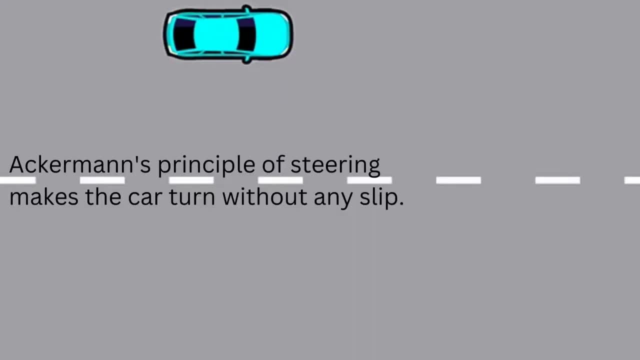 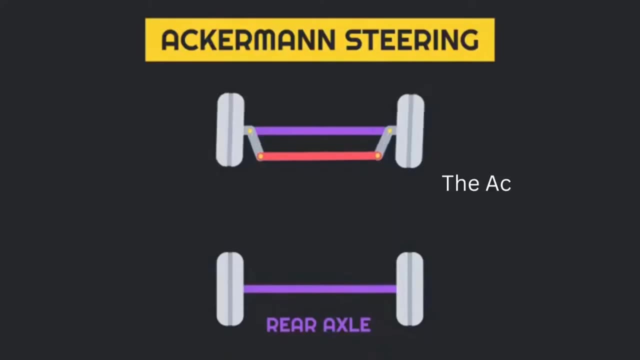 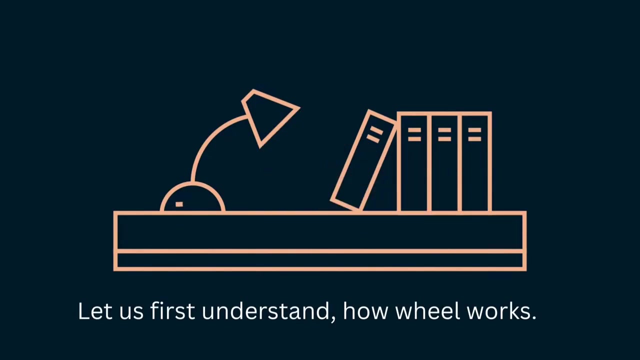 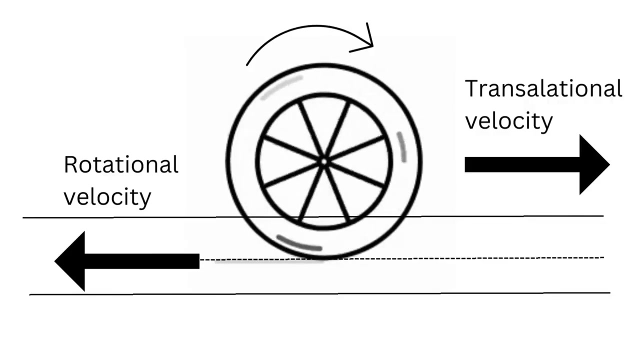 Ackermann's principle of steering makes the car turn without any slip. The Ackermann steering mechanism is a modified four bars linkage mechanism. Let's first understand how a wheel works. A moving wheel has two wheels. There are two different types of velocities. 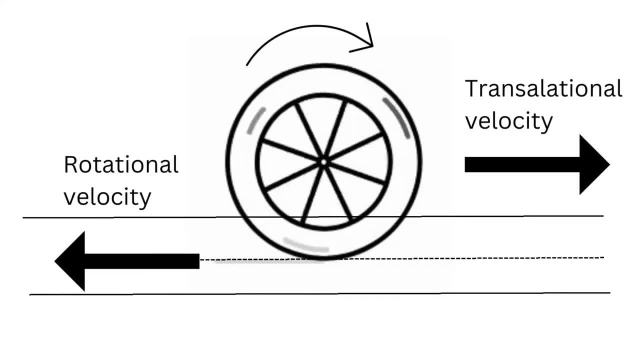 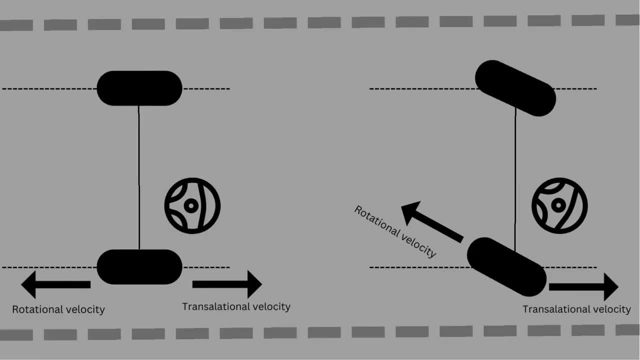 One is the rotational velocity and the other is the translational velocity. These both velocities are equal in magnitude but are opposite in direction, Hence they cancel each other. When the wheel has turned, the direction of the rotational velocity changes and there may be a possibility of slip. 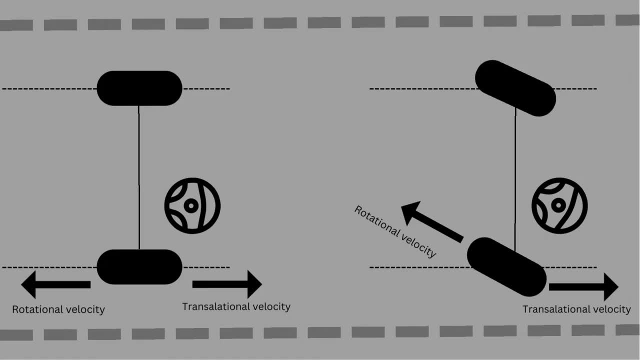 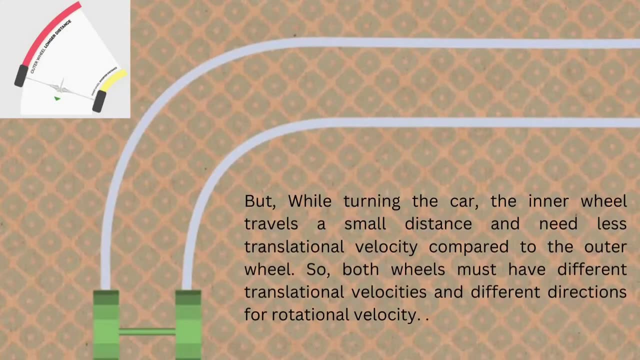 To avoid that slip, the direction of the translational velocity has to be changed. But while turning the car, the wheel has to be turned. The wheel has to be turned. The wheel has to be turned. While turning the car, the inner wheel travels a small distance and need less translational velocity compared to the outer wheel. 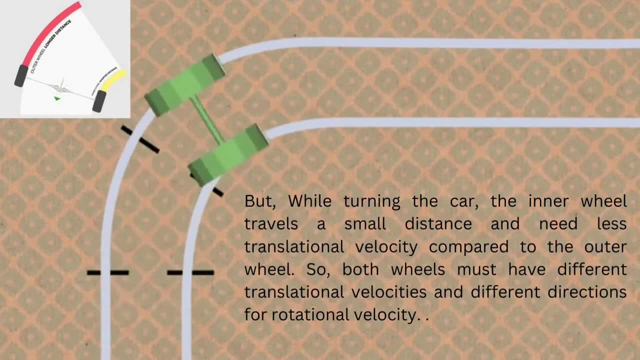 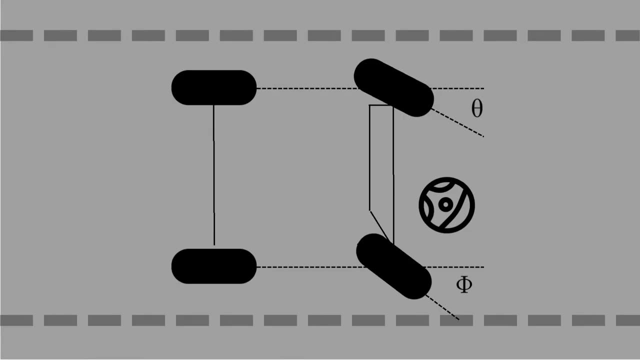 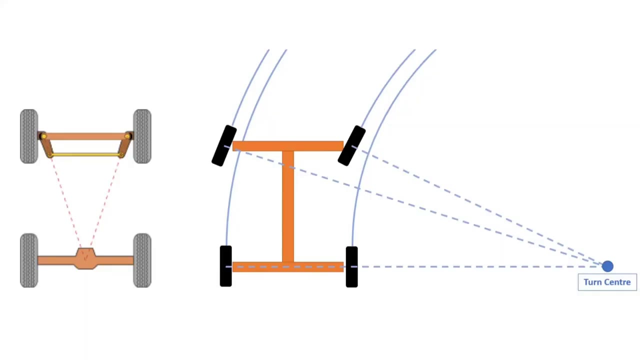 So both wheels must have different translational velocities in different directions for rotational velocity. This difficulty can be overcome by having different steering angles for two front wheels. The purpose of Ackermann geometry is to avoid the need for tires to slip sideways when following the curved path. 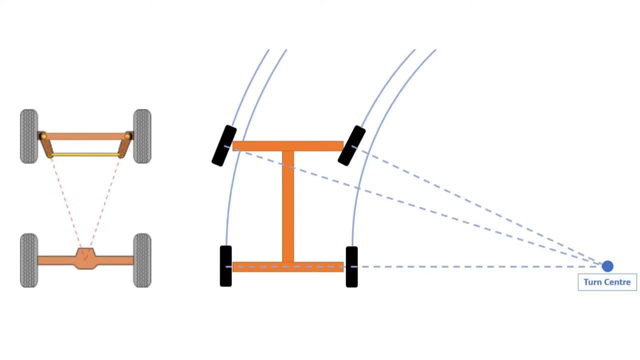 The geometrical solution to this is that all wheels shall have their axles arranged as radial lines which are spiked, puzzle-like, not slanted. Its rear wheels should be fixed with a cats causes. in these ladies heels single. as the rear wheels are fixed, the center must be on a line extended from the rear axle.